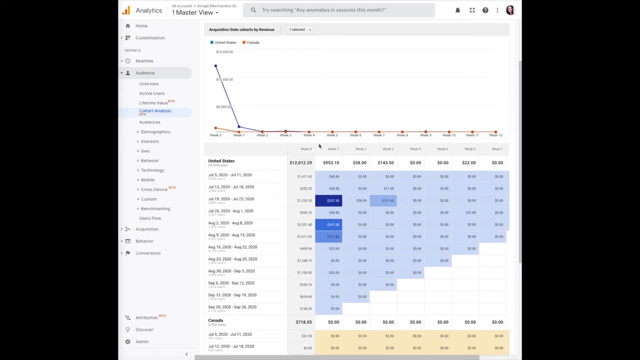 now we know we need to re-engage users, in week one, probably with a discount, and in week three, showing them new products that have been added or new products that they may be interested in, before they drop off completely If we're unable. 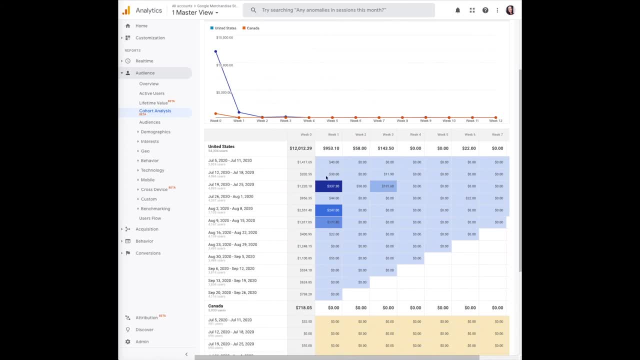 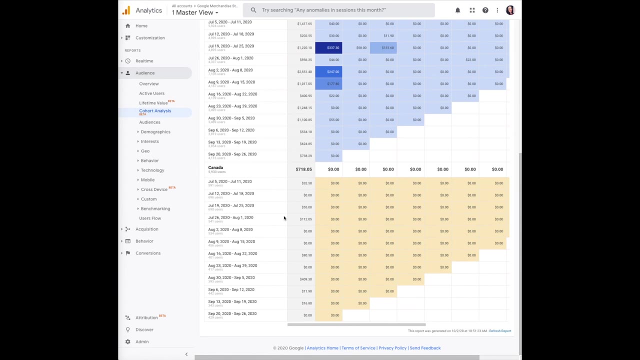 to recapture these lost customers. we know that in order to maintain the level of growth you want as a company, you need to acquire new users every three weeks Here in Canada we see, after that very first week we lose them completely. So we need to recapture in. 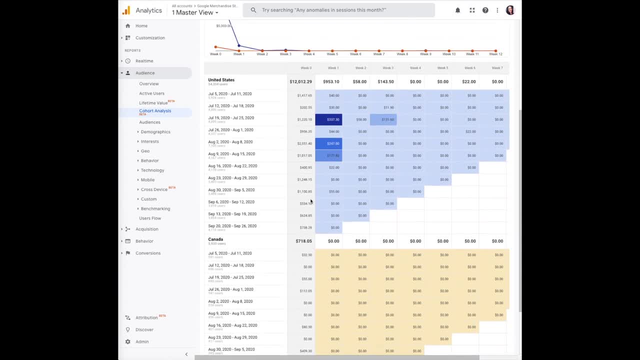 that very first week or otherwise. in Canada, in comparison to the US, we have to be gaining new customers every single week. 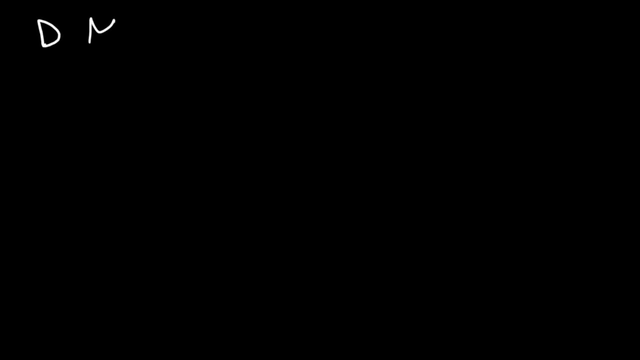 Now let's talk about how to convert DMS- that is, degrees, minutes and seconds- into a decimal in degrees. I like to think of an hour as being equal to one degree, and there's 60 minutes in one hour and there's 3,600 seconds in an hour. This will help you. 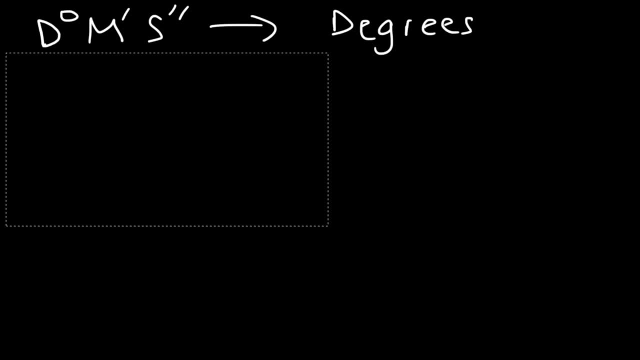 to remember what to do when you're converting DMS to a decimal in degrees. So let's say, if we have the value 45 degrees, 28 minutes and 32 seconds, Let's convert that to degrees. So here's what you need to do. 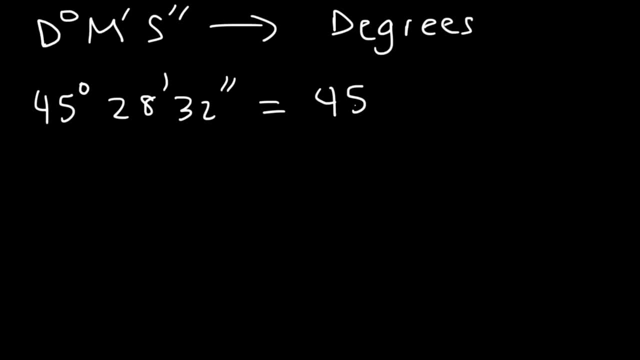 It's going to be equal to 45 plus 28 divided by 60.. Always divide the number of minutes by 60, because there's 60 minutes in an hour, Plus 32 divided by 3,600.. There's 3,600 seconds. 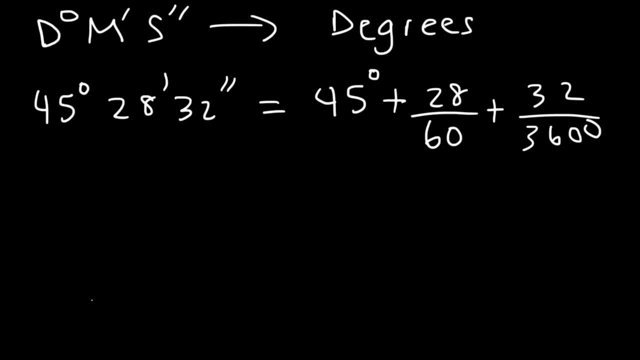 in an hour. so divide the seconds by 3,600.. And just type this information in your calculator and it should give you the answer. So if you're going to convert DMS to a decimal in degrees, you're going to have to convert.